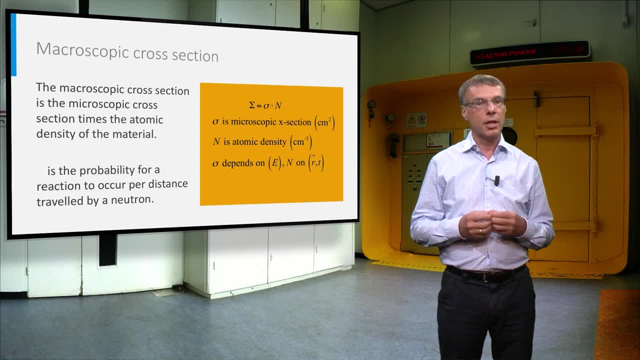 neutrons per unit volume and per unit time. Previously we have seen that a microscopic cross-section of a nuclide is the effective area of the nuclide for interaction with neutrons. You can easily imagine that the number of reactions of a neutron beam with the atoms. 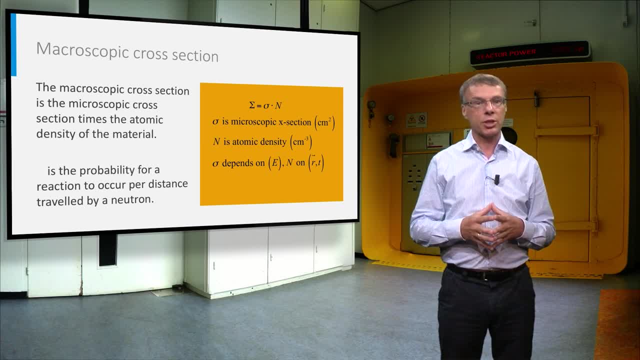 in a material will be proportional to this microscopic cross-section, but also to the atomic density of the material. The product of these two factors is called the macroscopic cross-section of the material, And we will use this macroscopic cross-section on the next slide. 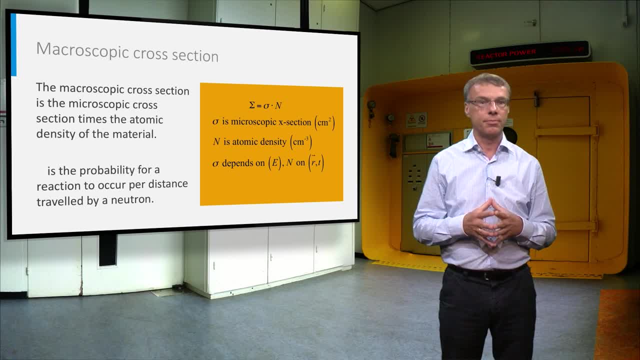 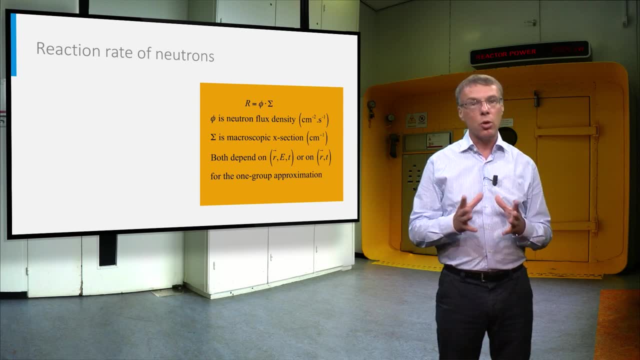 to calculate the reaction rate density in a material On the previous slides we have seen that the neutron flux density is the total distance travelled by all neutrons per unit volume and per unit time, and that the macroscopic cross-section is the interaction rate per unit distance travelled. 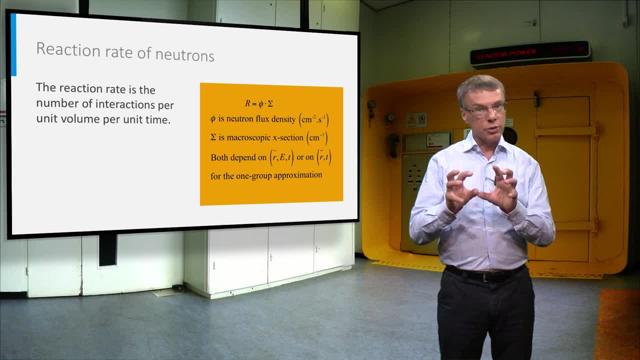 by the neutrons. This means that the product of these two factors gives the total number of reactions per unit volume per second. This parameter is called the reaction rate density. This parameter is called the reaction rate density. This parameter is called the reaction rate density. 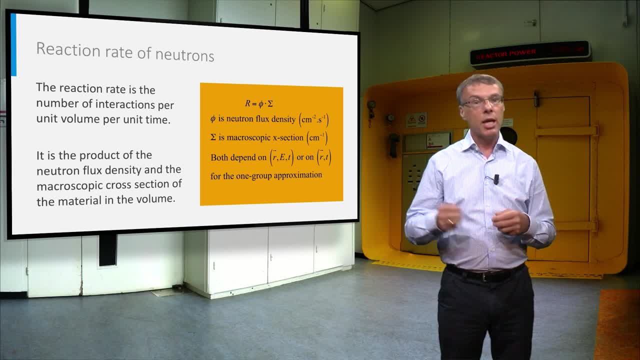 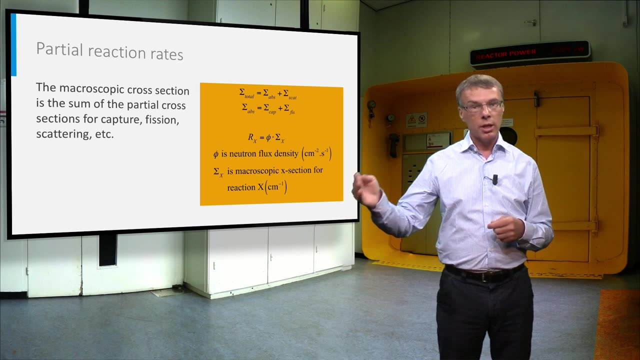 Because the neutron flux depends on space, energy and time, and because the macroscopic cross-section typically also depends on space and energy. the reaction rate density is also depending on these parameters, Because the macroscopic cross-section can be split into the individual contributions. due to neutron capture, fission and scattering. also, the reaction rate can be subdivided in these two separate contributions And the units of these partial contributions are the same as for the total reaction rate and the sum of all partial reaction rates is equal to the total reaction rate. 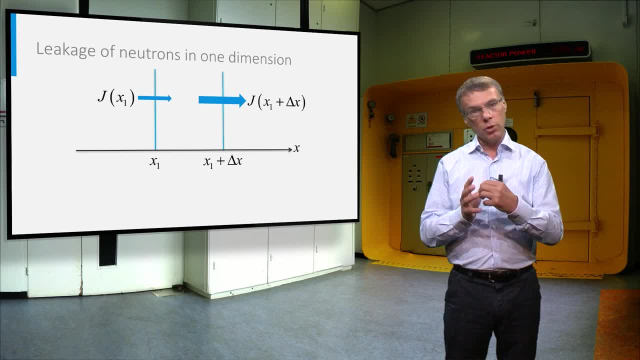 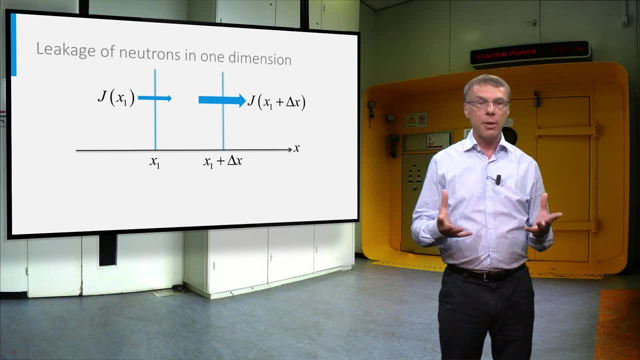 Now we will derive an expression for the leakage of neutrons from a volume element. For simplicity, we will derive this expression in one dimension. first, Imagine neutrons streaming from left to right. If the neutrons streaming out of an element, delta x, are in the same direction as the neutrons streaming out of a volume element. 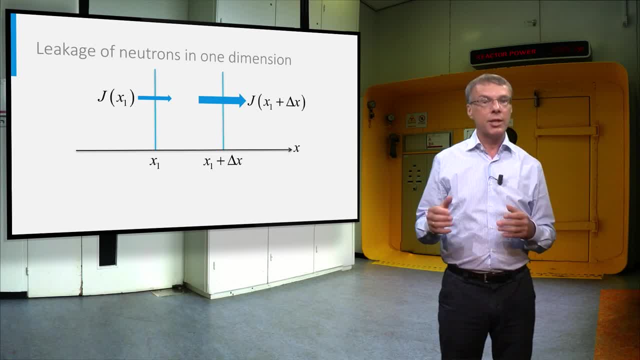 it is larger at the right boundary than it is at the left boundary, there is a net positive outflow of neutrons. The leakage per unit size of the element delta x is equal to the derivative of the neutron current called J. 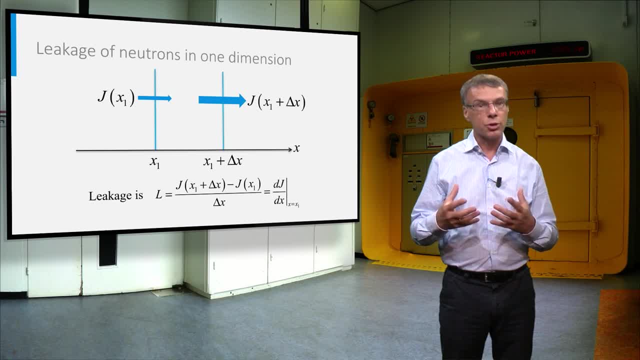 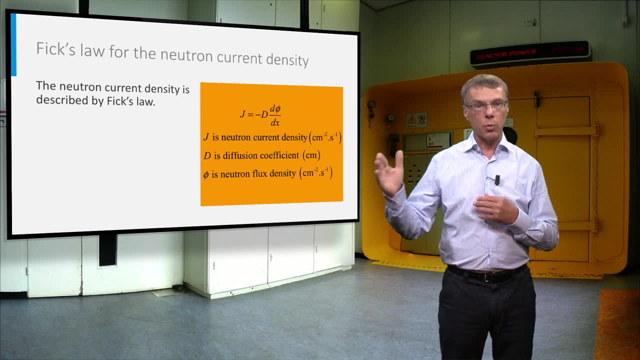 On the next slide we will derive a simple expression for the neutron current based on Fick's law. Now we will derive an expression for the flow of neutrons from one region to the other. In the fusion theory, the transport of particles is described as being proportional to the gradient of the. 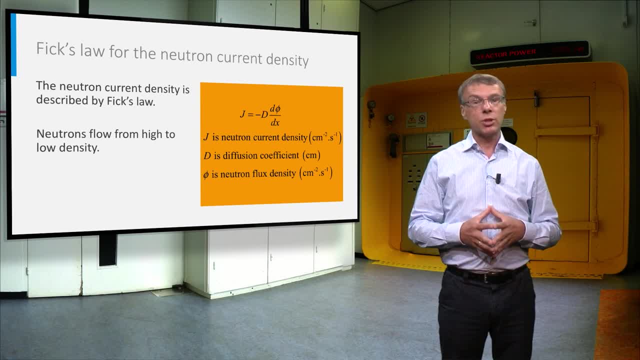 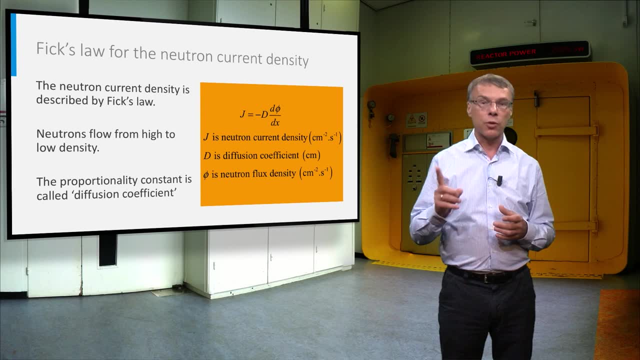 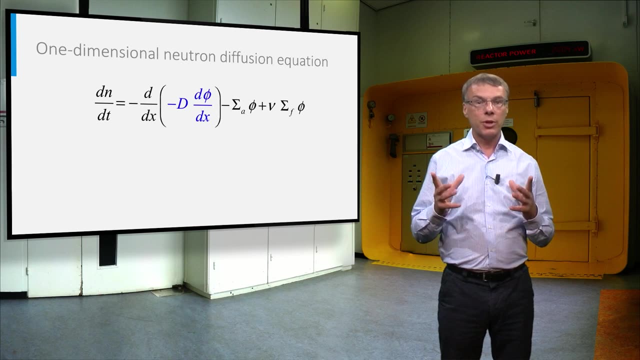 particle number density. In reactor physics this would translate into a neutron current density that is proportional to the gradient of the neutron flux density. The formula for J gives the expression in one dimension, namely in the x-direction. We will now derive a neutron balance equation in the fusion theory by looking at each loss. 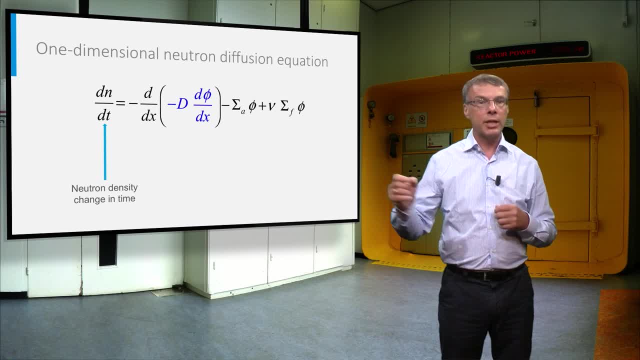 and gain term in the unit volume. Let of the balance is a time derivative of the neutron density. If this time derivative is zero, we have a stationary neutron flux. otherwise it is increasing or decreasing in time. The first term on the right hand side describes the flow of a neutron in the x-direction. 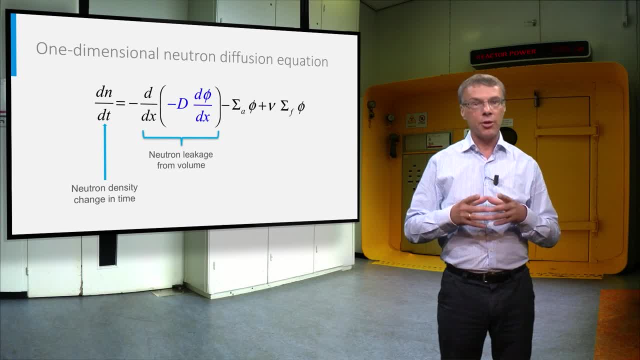 We would have similar terms with Y and Z in a 3D problem. The term in blue between brackets is a neutron current density. in the 3D problem, The actual pattern of the eden-artstand turns out to be a negative slope. which is characterized by theradas of turn objects and moving zas: gravity, x- rad, Details of the added j's as the constant других of x-Park supersede these nessaltic terms. physical of anrahac más these M74 touch RT, freeze 1994, and naming the bonds between R and 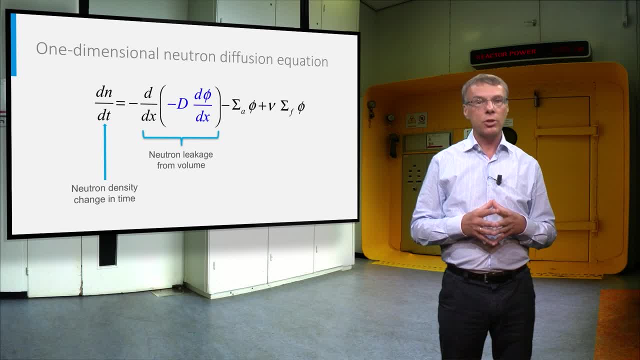 fusion theory using Fick's law. Note that we have two minus signs here, because a leakage is counted as a loss term in the balance equation, which adds another minus sign in front of it. The second term on the right hand side is the absorption rate of neutrons, which is 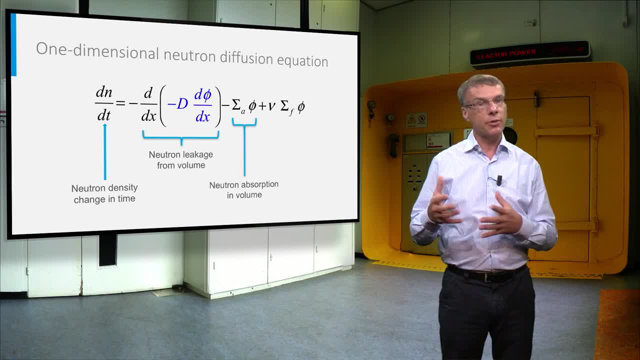 also a loss term and which has therefore also a minus sign in front of it. And the third term on the right hand side is the fission neutron source term. This is equal to the fission rate density multiplied by the average number of neutrons. 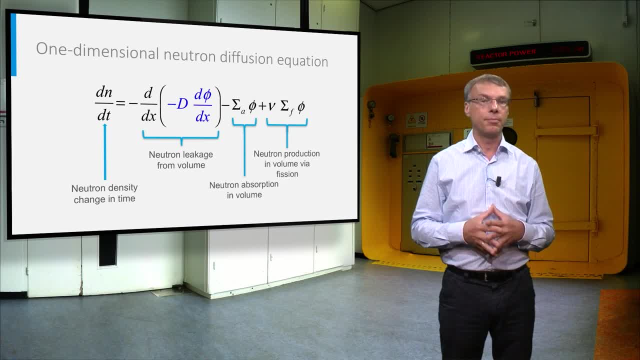 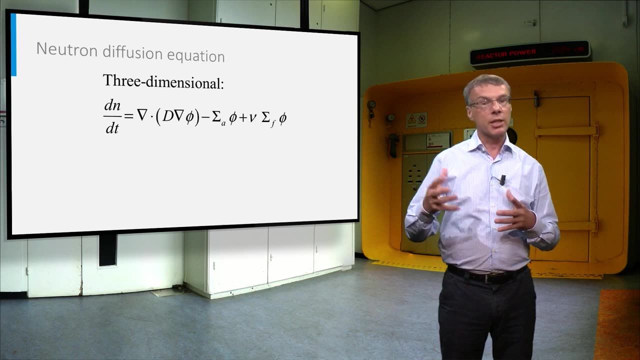 released in a fission event indicated by ν. For most reactors using uranium as a fuel, ν has a value of about 2.5.. This equation shows the same expression for the three-dimensional case where dΦdx is now replaced by the nabla operator. 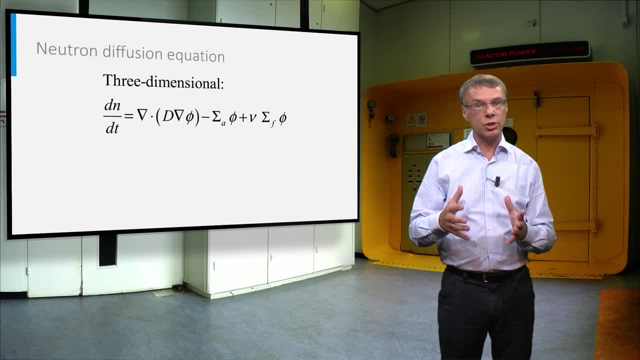 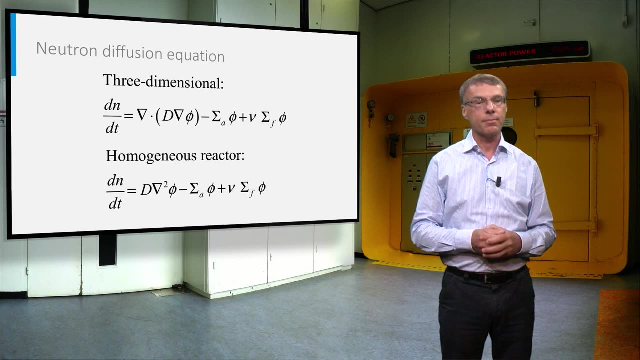 Nabla stands for the three-dimensional derivative in all three directions: x, y and z. If we would have a homogeneous reactor core, the diffusion coefficient would not be spatially dependent anymore and the equation would become as in the bottom line. There is one important step to make.